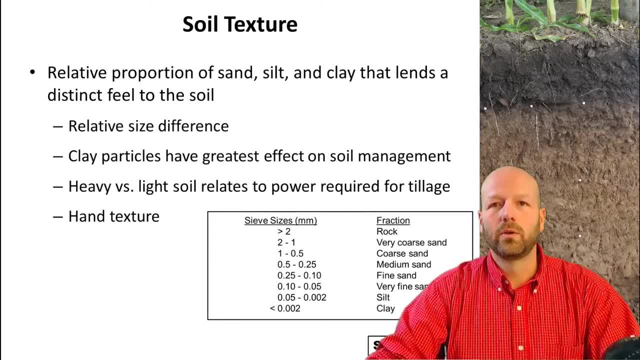 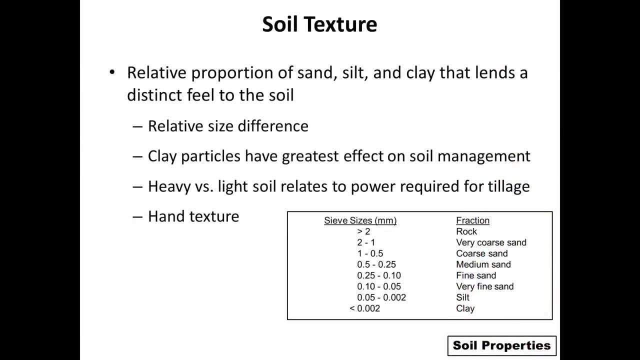 As we're breathing right now. So, talking about the solid phase In the mineral portion, we know that that's composed of what we typically call sand, silt and clay, So this is another way to refer to this. Many times we call it the soil texture. 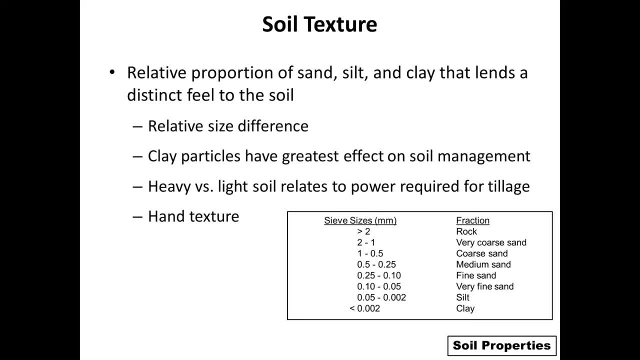 And what the soil texture actually is is just a relative proportion of the sand, silt and clay in a different soil. And if you get a soil sample and kind of rub it between your fingers you can kind of figure out and feel you know. 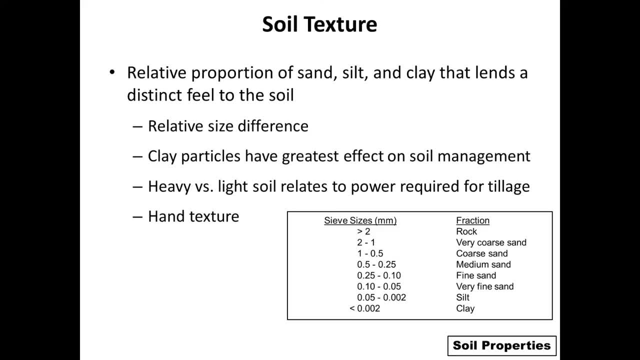 that relative proportion, that feel. So that's actually called the feel method. A lot of times you might hear soils being referred to as heavy or light And that's not related really to the density of the soil or the weight of the soil. 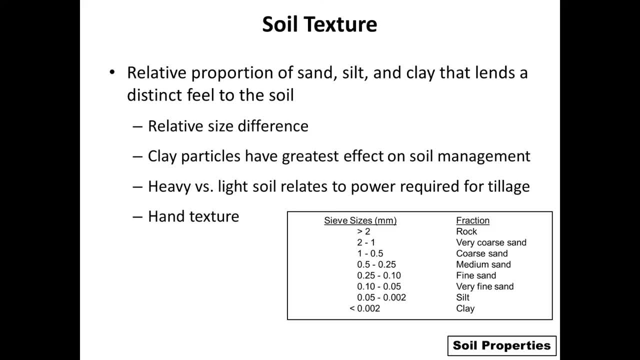 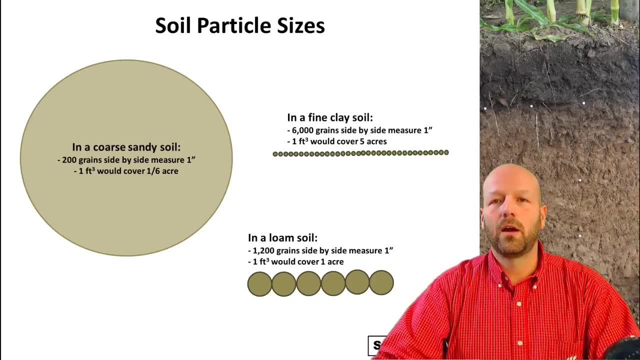 but more to the power requirement- And we can talk about this in a little bit more detail in a second, Talking about the different salt particles. a lot of times when we're thinking about sand, silt and clay, we don't realize that they actually do have. 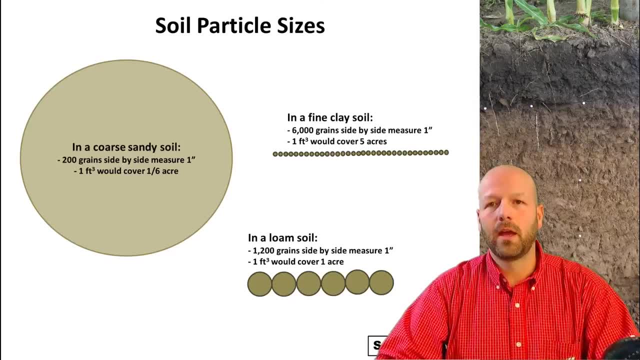 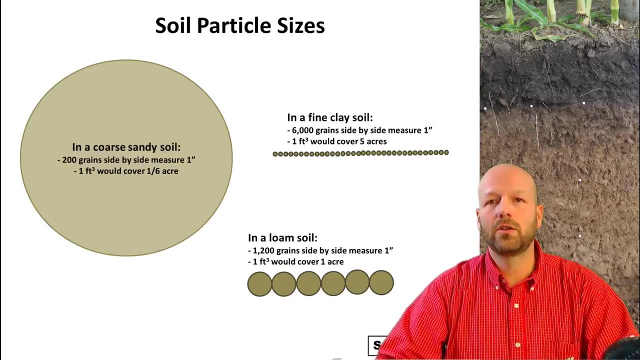 a wide range of properties and they're very different. Sand, for example. sand particles are much larger than silt and even clay particles. It would take 200 grains of sand to cover one inch of distance if you were lining them up side by side. 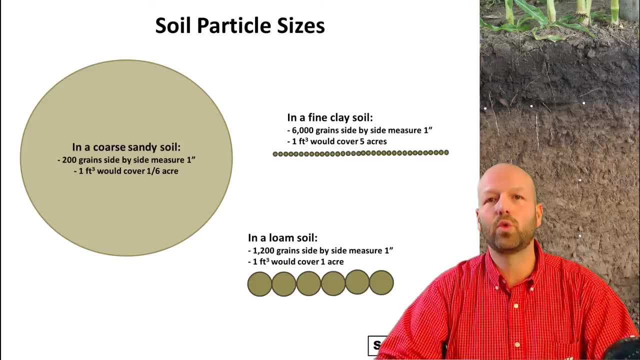 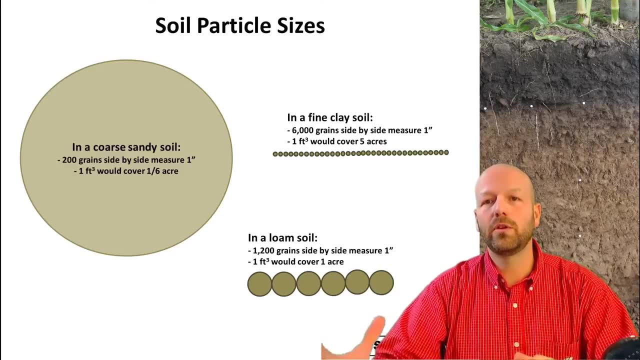 The same distance you would need to cover the same distance. you would need 1,200 grains of silt and you would need 6,000 grains of clay. So clay are much, much smaller. Another way to view this is also to how much. 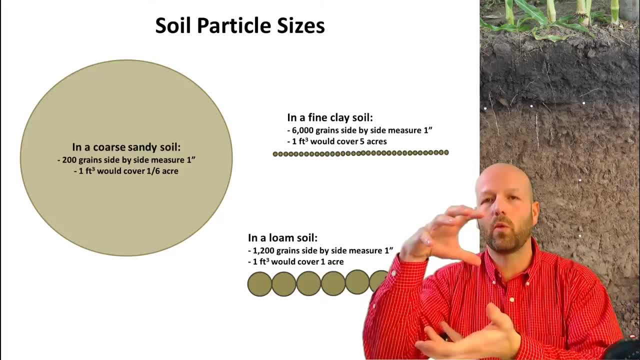 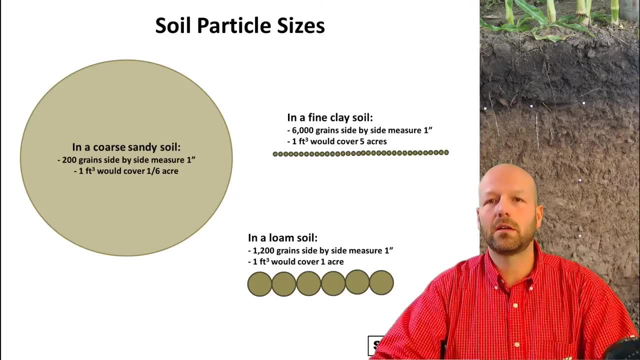 volume in the surface area of this particle. So if you were to get one cubic foot of sand and spread it around on one layer, that would cover one sixth of an acre, So just not even an acre. If you were to do the same thing with loam. 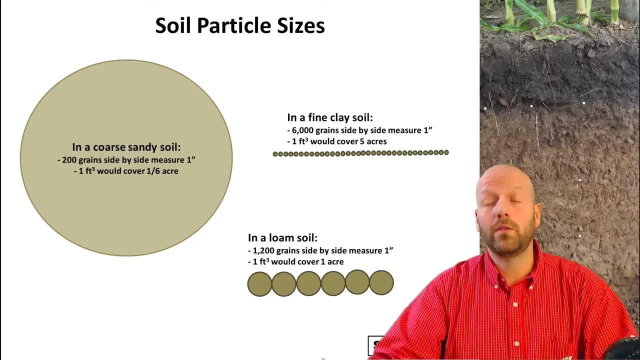 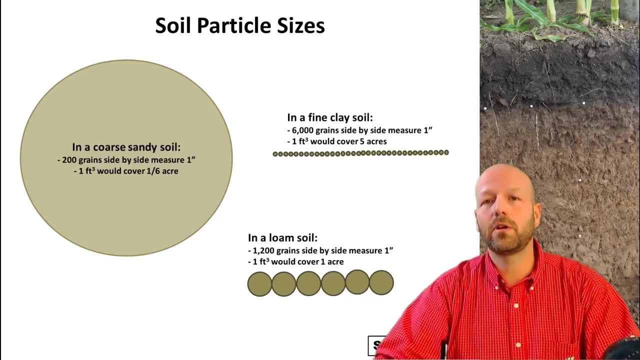 that would cover one acre. If you were to do the same thing, filled up one cubic feet of soil with just clay, that would cover five acres. So that gives you a big idea on the wide range of particle size and also their specific surface area. 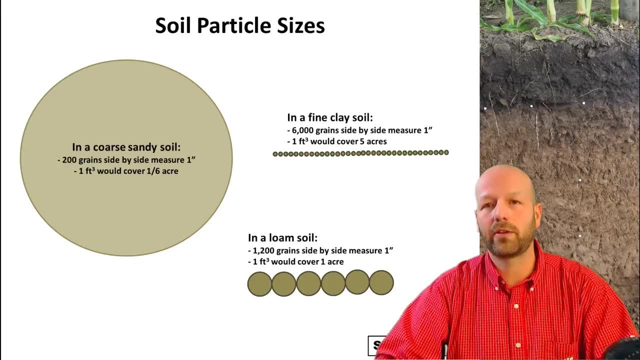 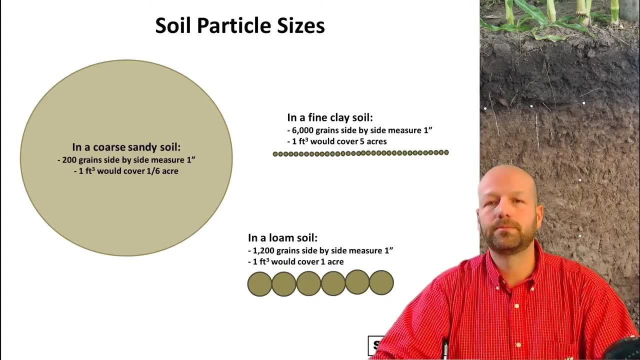 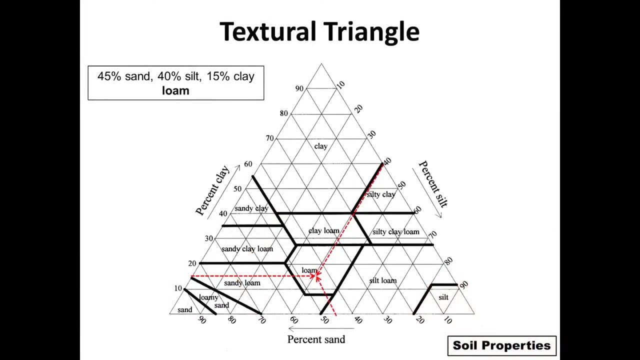 or the surface area of each particle, With clay having the greatest surface which imparts a lot of important properties to soil, followed by the silt and then the sand. So we talked about the field method or the texture of the soil. So you might recall the textural triangle. 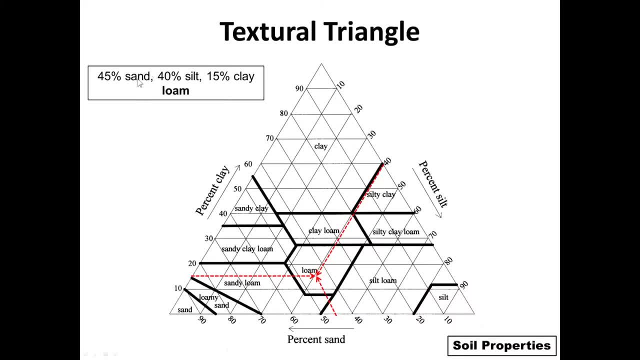 So you can see here in this figure, Here's an example that I have here on this box here, of a loam, And we have that. that loam is 45% sand, 40% silt and 15% clay, And so here's how we arrived to this number. 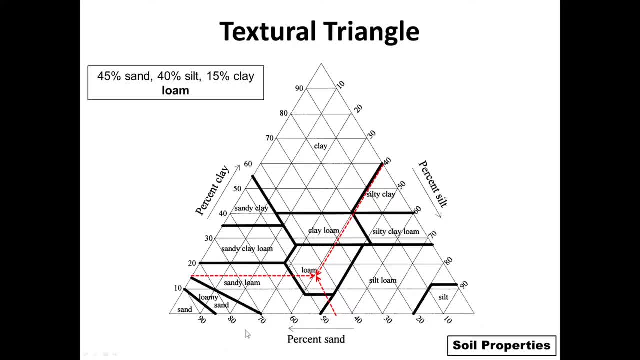 So here's the sand. So on the bottom we have the sand axis, if you will, And so we looked here at 45% and we go up. Then we can look at the silt, which is, in this case, 40%. 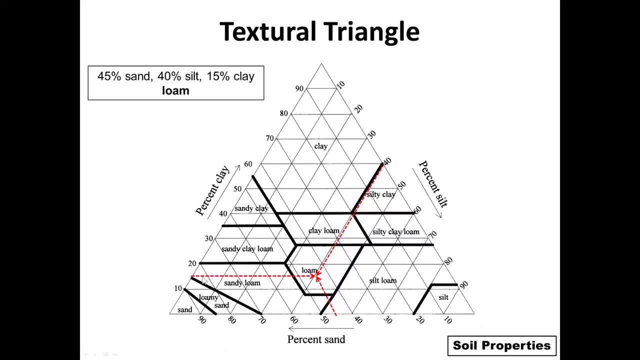 And then we kind of go down and meet where that sand percentage was And then look at the clay, which is a 15%, And we can see that that sample falls in the loam range. as far as a texture or a textural triangle, 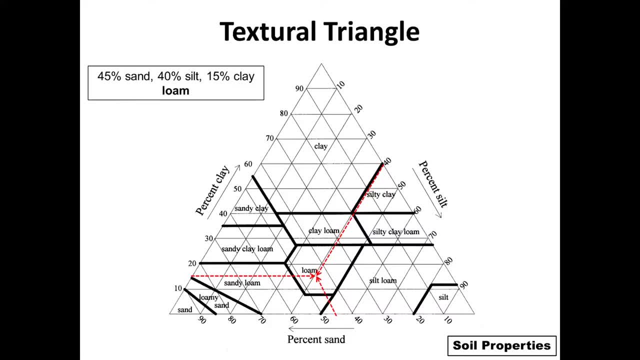 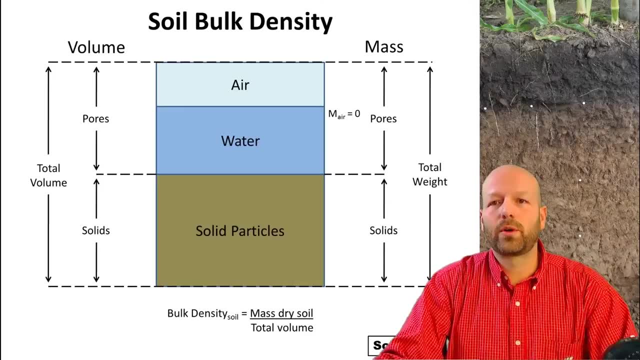 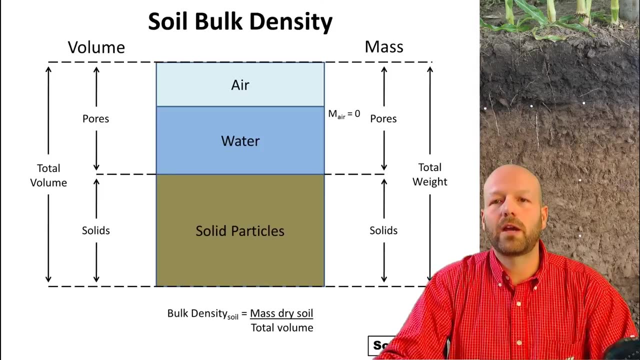 So this is how you use a textural triangle to figure out different textures for different soils. if you know the particle size distribution. Soil bulk density is another important soil property. Essentially, what we're looking at is the proportion of dry soil, or the mass of dry soil divided by the volume of the soil. 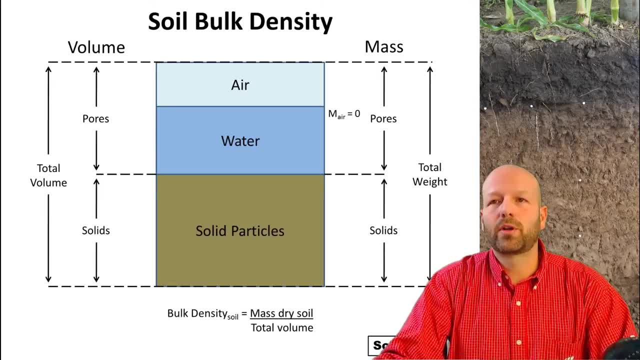 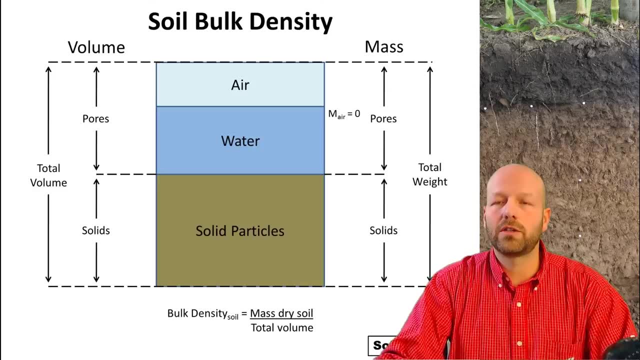 as we can see in the equation at the bottom of the slide, And this is an important property because it gives us an idea on the proportion of pores, And the pores are very important, as we will see, for a lot of water relations and a lot of properties in the soil. 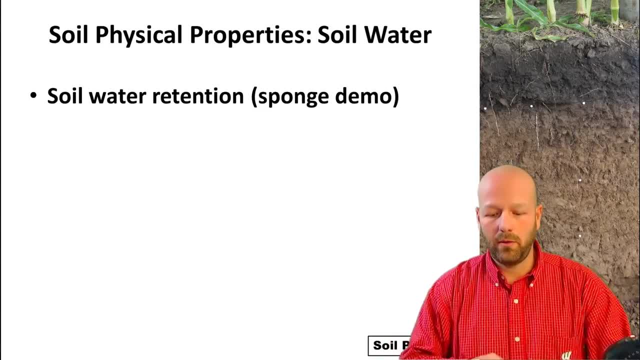 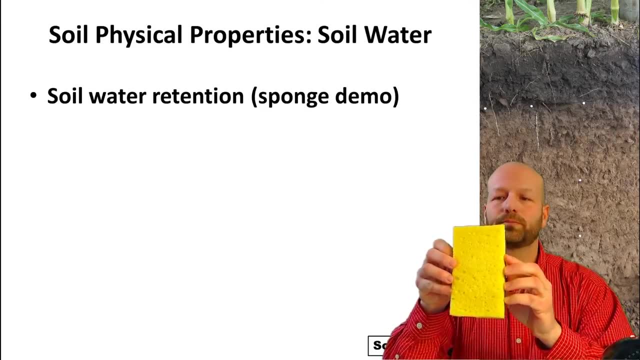 So now I'm going to show you a little demo here, And I call this the sponge demo, And what this is actually trying to attempt is to show you how water is held in the soil. So I have a sponge here, just a regular cleaning sponge. 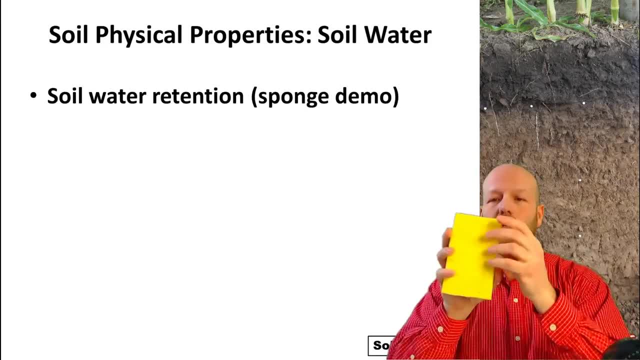 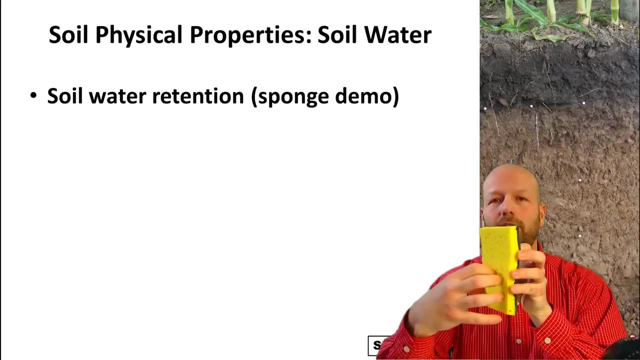 which is fairly dry, as you can see, And this sponge, if you think about soil, it's a good model for soil, So it has a solid face and it has porosity to it, So I'm going to put it inside a little bowl I have here with water. 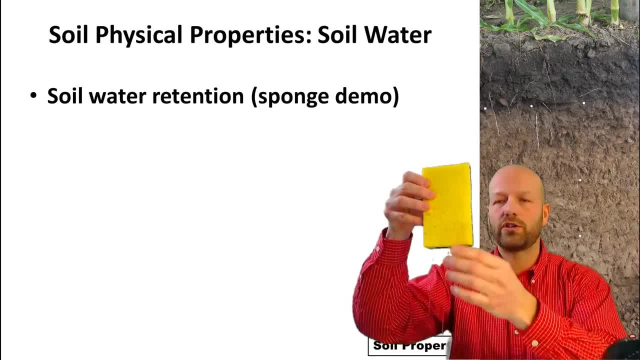 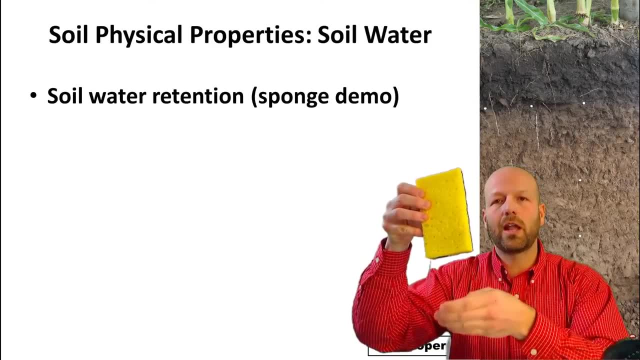 And what happens, as you can see here, is that water is dripping out of this sponge. So this is the water that is held in the larger pores, Similarly in soil, after a good rainfall event, we get this water that drains out. 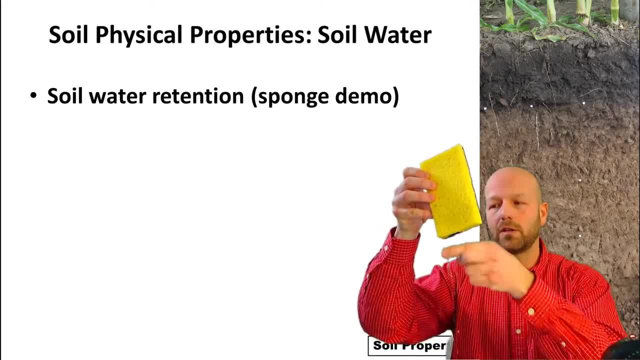 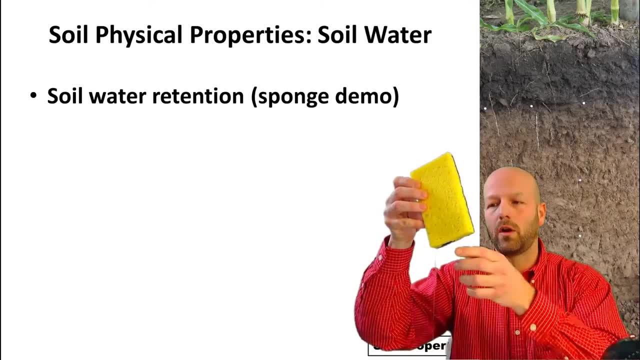 What's happening is that gravity, the rotational force of the air, is actually pulling this water out of the sponge. in this case, Same thing happens in the soil after a good rainfall, where the larger pores drain due to gravitational forces, And this is what we call the gravitational water. 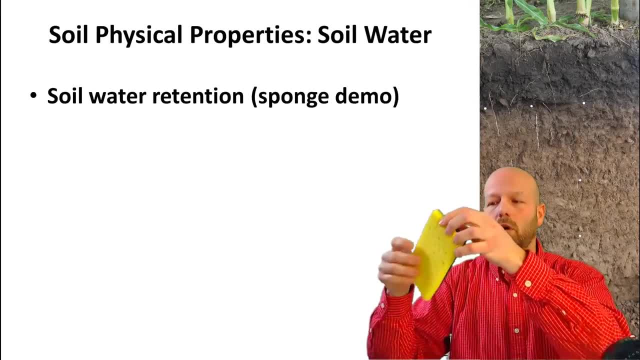 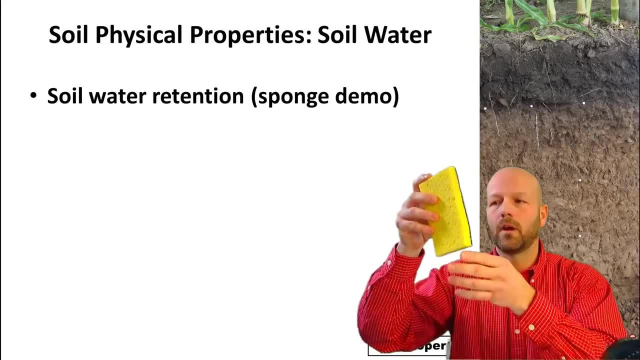 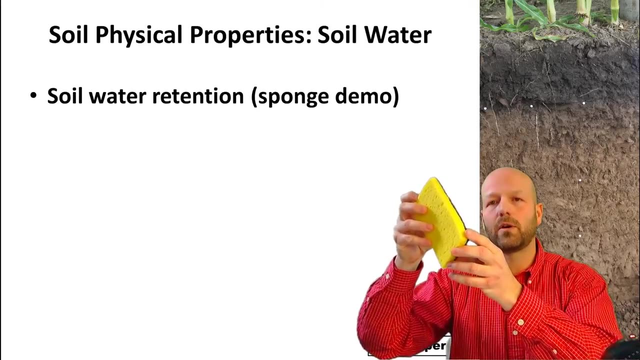 So this would be under saturated conditions. So once that flow of water stops that gravitational water, then we can see that there's no more water coming out. This is what we would call field capacity in a soil. So the way we define that in soil is: 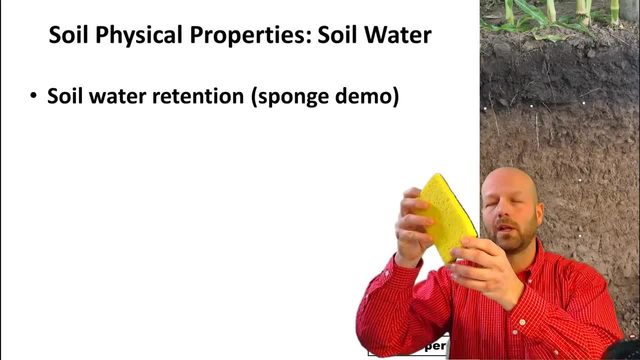 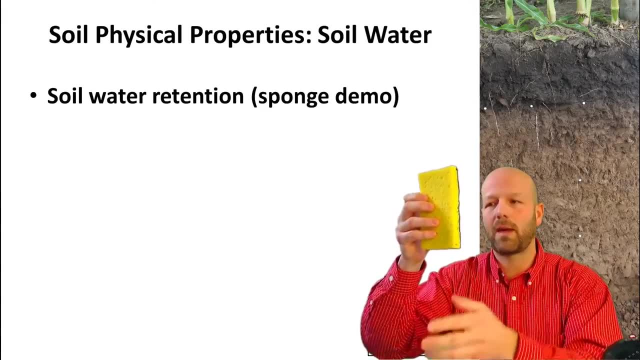 after a good rainfall and the soil is saturated, we let that soil drain, let that gravitational water escape for 24 to 48 hours, and that's what we call field capacity. So it's more or less what's happening here. So what happens is that the larger pores have drained. 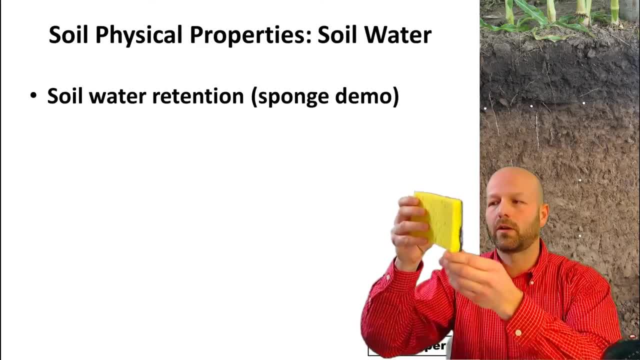 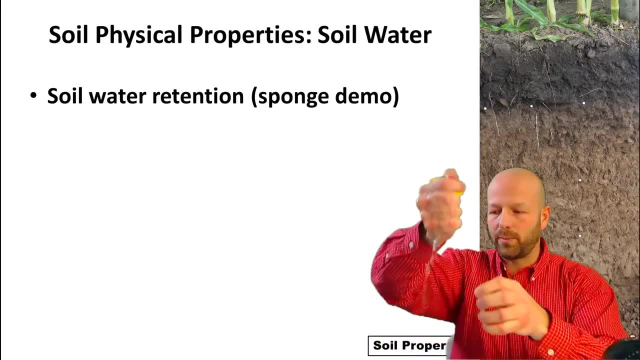 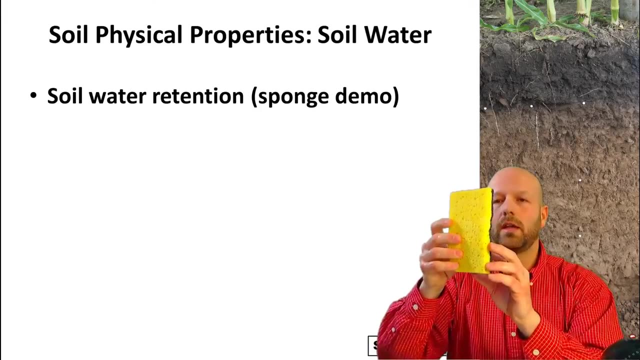 They cannot hold water under just regular conditions. And now we are at a field capacity. So if I go and squeeze the water out of this sponge- so I'm mimicking, let's say, the plants extracting water out of the soil- then I have the sponge where it's not completely dry. 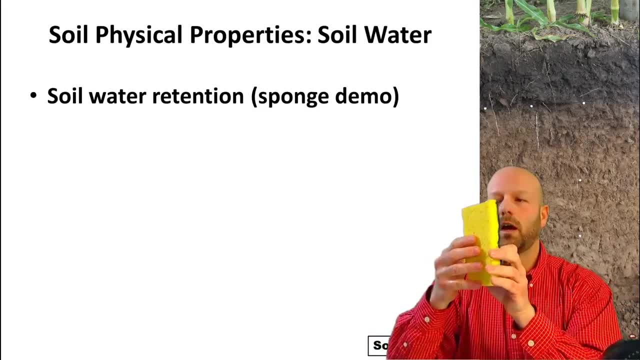 but it's fairly dry. There's still some moisture in the sponge, So the same thing would happen in the soil. when a crop is taking up the water, It will take a lot of the water out, but then there's still some water in there. 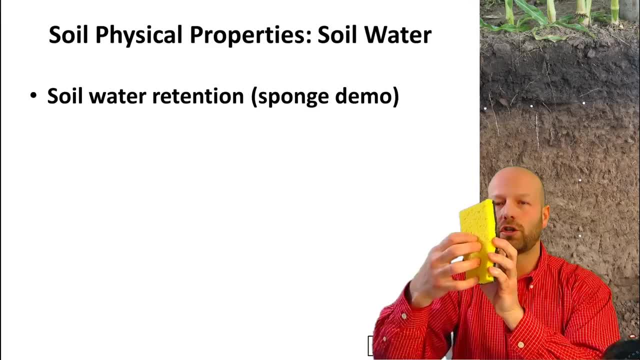 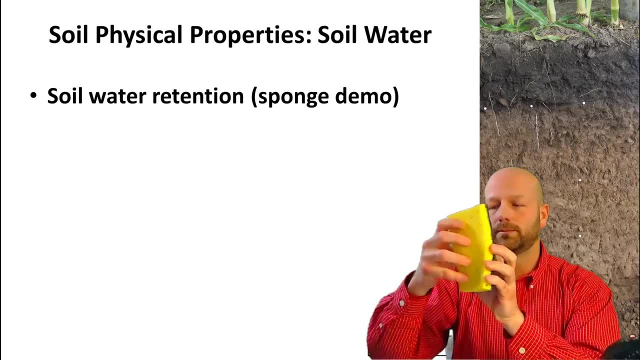 But the water in here is held very tightly. Water in the soil is held under a suction and plants cannot extract this water anymore. So this would be analogous to what we call the permanent wilting point in soils. So again, this is all relating the pore space. 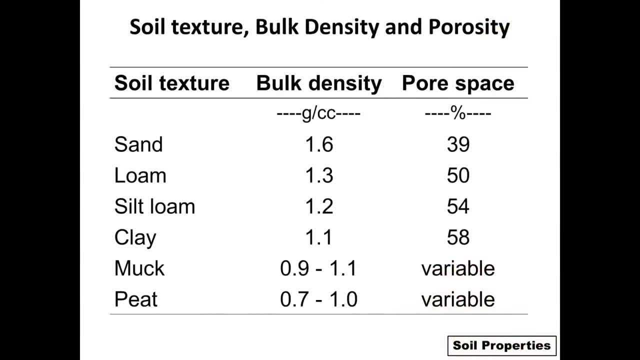 and the porosity in soils. And here's an example: looking at just some relative soil textures and then looking at just an average rule of thumb bulk density and what would be their pore space, And you can see that sands- even though sands we usually have the idea that hold a lot of water. 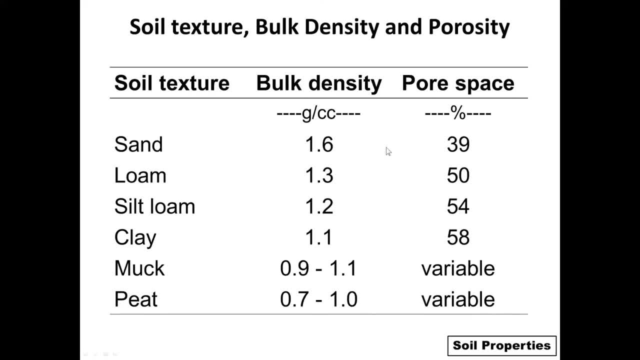 or have a lot of water in them, a lot of porosity to them, they actually do have less pore space relative to a loam, a silt loam or even a clay, And again this goes back to that surface area. 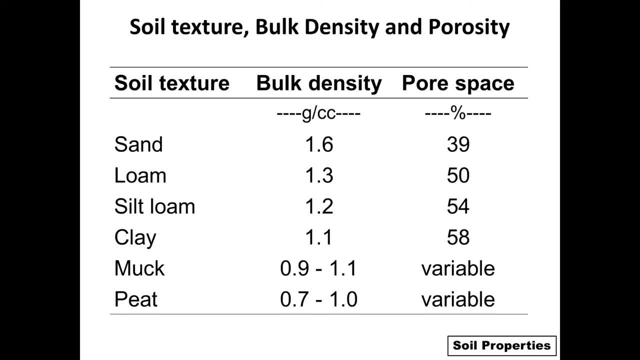 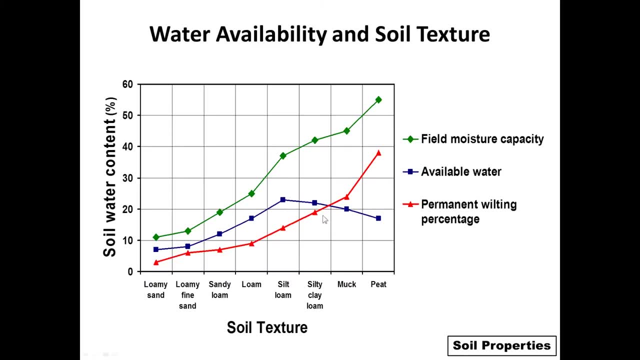 a specific surface area where a clay soil has a lot of spaces and has a lot of surface for that water to attach to, If we're looking at the water availability of soil and the different textures. so what's the impact of the texture on water availability in soil? 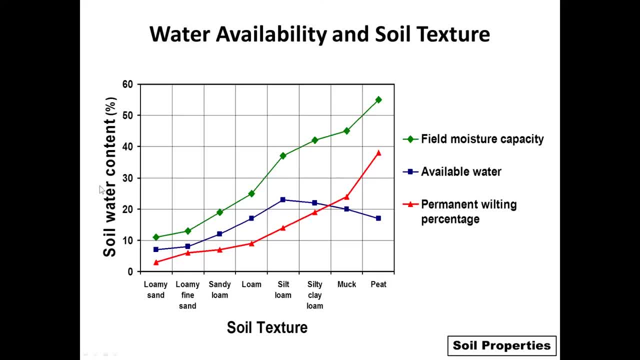 we can see here in this figure. So we have on the vertical axis we have soil, water content, and then on the bottom axis we have the different textures. We have different soil textures, going from loamy sand all the way to mock and peat. 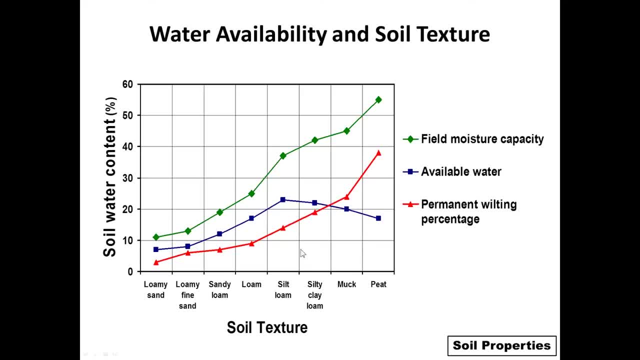 The green is the field moisture capacity, The blue line is available water and then the red line is the permanent wilting point. So, at field capacity, remember the sponge model. that's actually. after all, the gravitational water has flowed out of the soil. 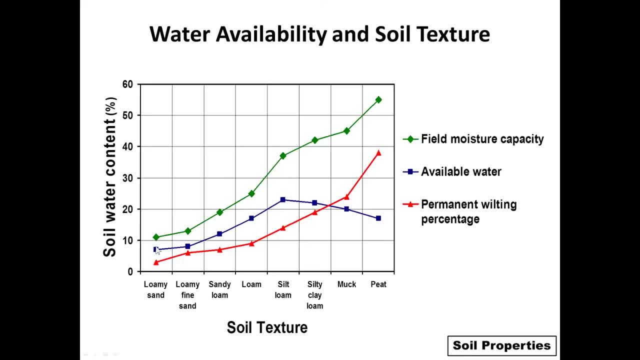 We can see that coarser texture soils. so the sands and the loamies are going to have less water. So they have a lot of big pore space so that water flows out very easily, But they also have less porosity. 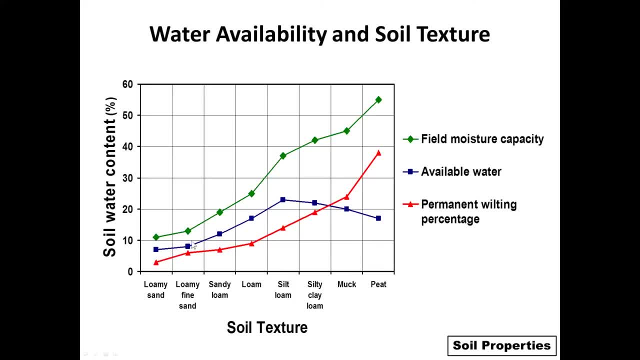 if you recall. So they also by the same way, then they're also going to have less available water. So if you look at this blue line and we're trying to find out what soil has the most available water, we see that a silt loam actually. 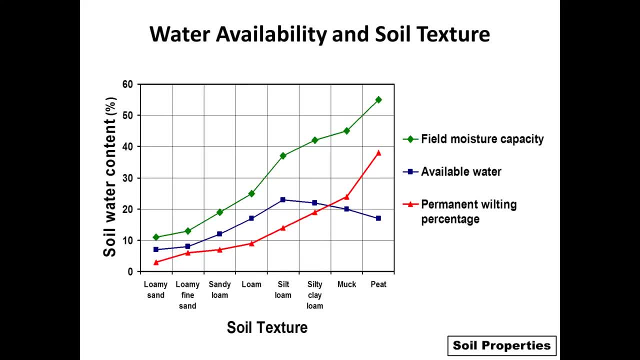 typically has the most available water. However, we know that clays can hold a lot more water. And why is this? Well, remember we're talking about plant available water, So clay does have a lot more pore spaces, but water in clay soils. 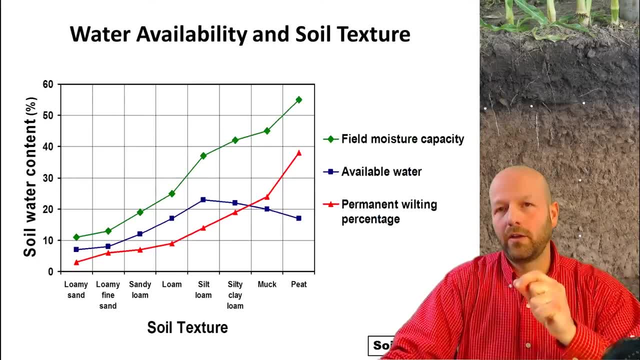 are held under a lot of suction, and it's held very tightly to the soil, so much so that plants have a really, really hard time extracting that water out of the soil, So that water is not truly available for the plants Where a silt loam has actually the best proportion. 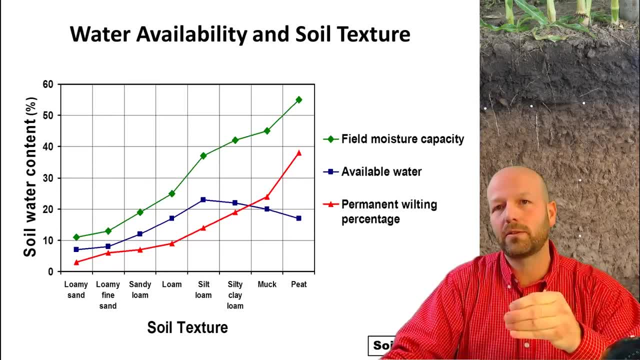 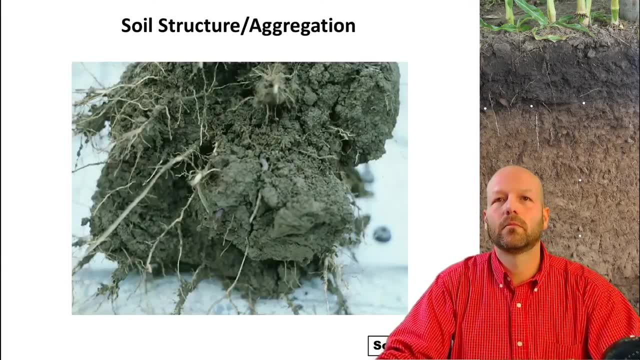 if you will, or the best composition, and it has a lot of pore space and it doesn't hold that water. and it doesn't hold that water so tightly that the plants cannot extract it. Now, going a step further, we know that sand, silt and clay particles 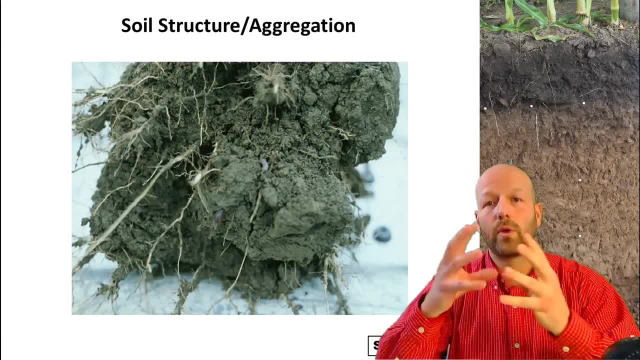 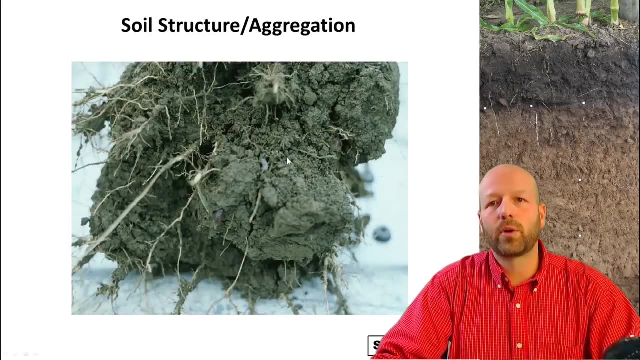 are not just floating around and existing by themselves on the soil. They form what we call aggregates, And here in this picture we can see an example of the aggregation. We know that aggregation is very important for water relations, for root growth and all sorts of different things. 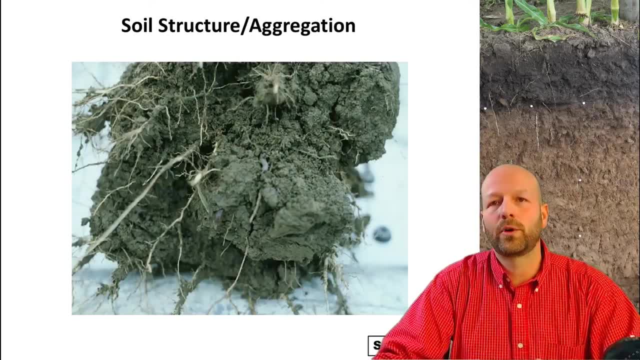 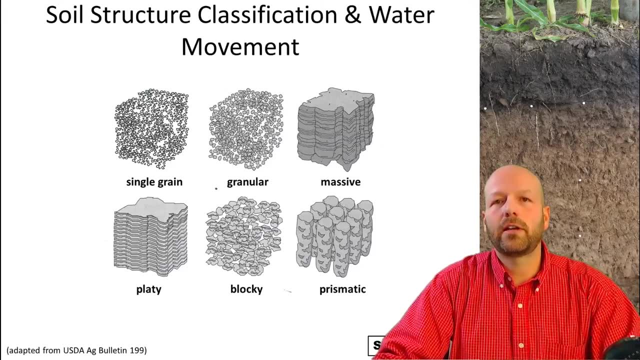 So let's talk about aggregation here and soil aggregates in a little bit more detail. So when we're looking at soil structure, classification or different aggregates, we see what we call a single grain. so that would be your sands, then granular. 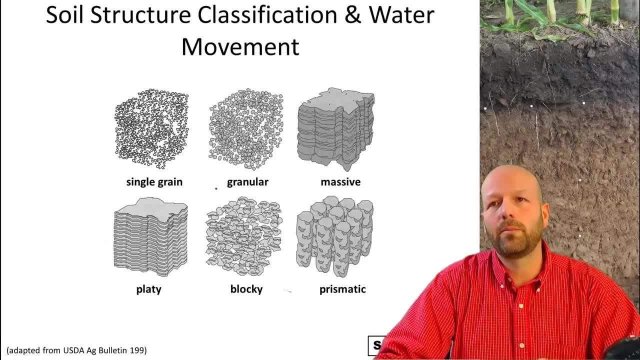 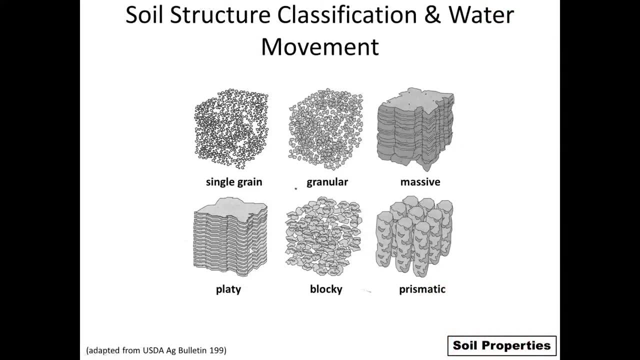 so then we have sand, silt and clay particles that are clumping together. We can have something like a massive structure. that would be something like a compacted soil, platy, blocky and prismatic When we're looking at structure. 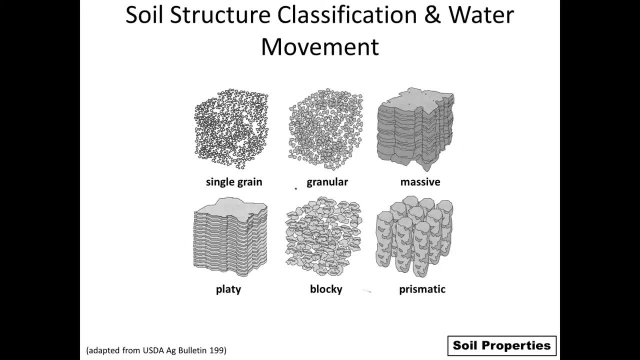 different soils are going to have different structures depending on how they're managed and what have not. But also when you look at a soil profile, as you go down in the profile you see that the structure of the soil changes. So typically deeper in the soil profile. 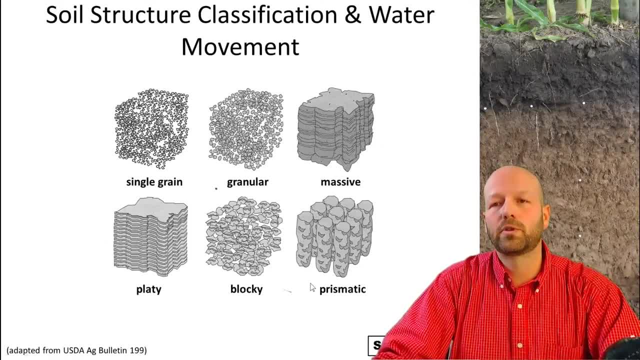 you'll see more of the columnar or prismatic type structure, where, towards the surface, you'll see more of the blocky or granular type structure And then, where you would encounter the massive would be under compacted conditions. That could be either surface or subsoil compaction. 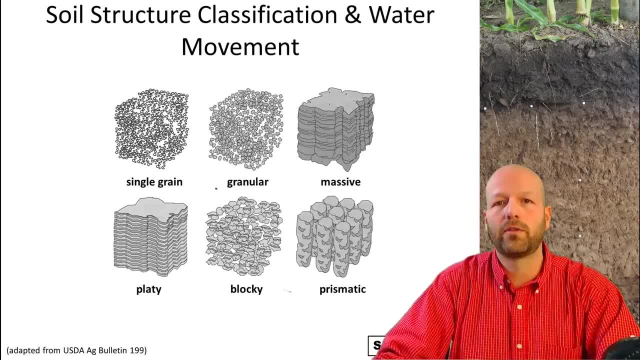 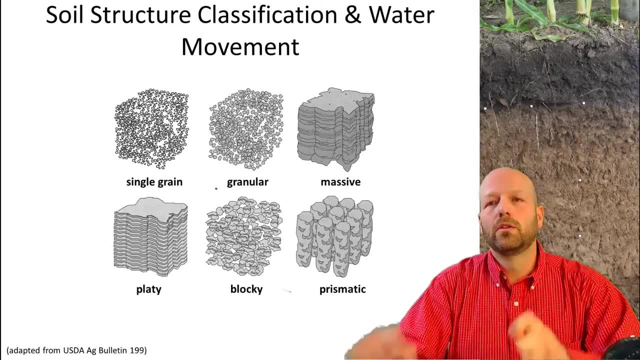 so you could have that either on the surface or lower in the profile And then the platy. you will find that over time it's also sometimes typical of compaction or some other soil issues. So if you're thinking about soil structure, 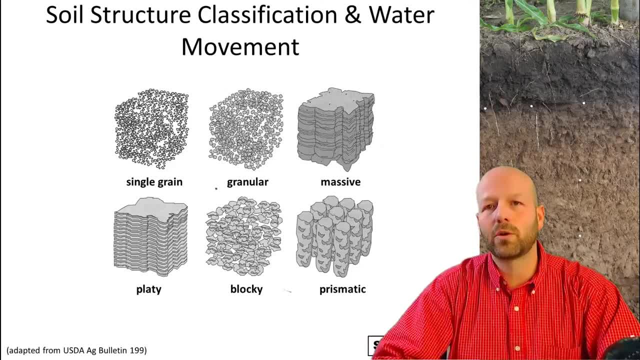 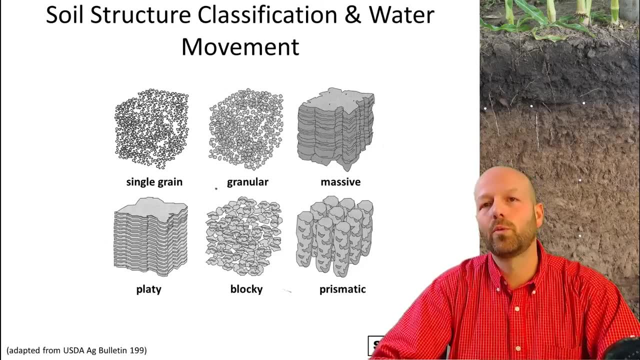 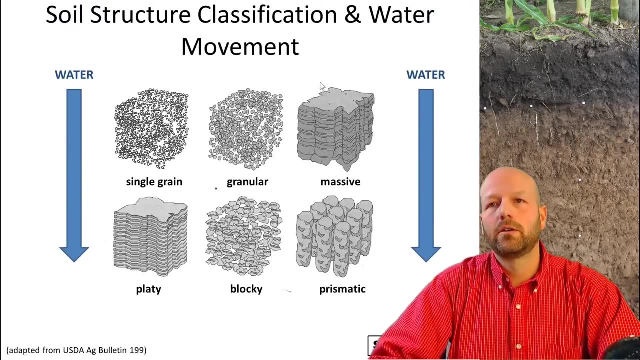 and then we're kind of moving that along with water movement in the soil and water relations. where do you think, looking at these different structures, water will flow more freely. So imagine water flowing through those different aggregates, So obviously massive and platy structures. 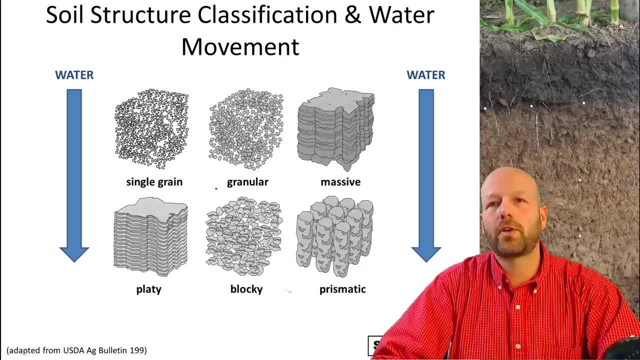 are going to restrict water flow. Water is actually going to flow fairly well through granular and blocky. but think about water. If you're a little water molecule trying to go through all these particles, do you have to take a lot of turns? 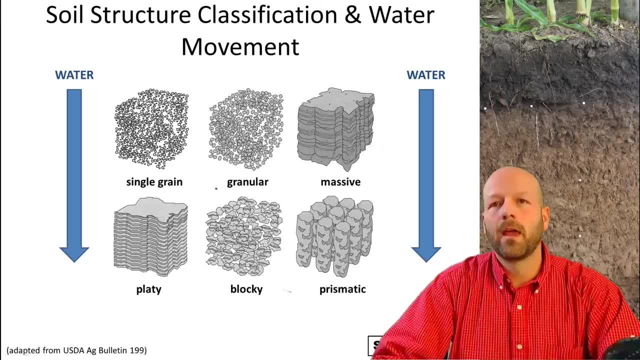 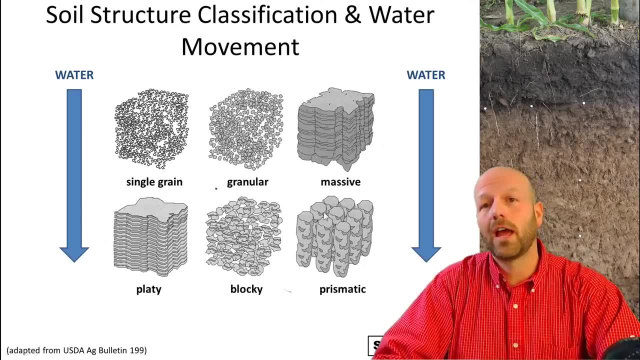 and zigzagging to get down. That's what we call tortuosity, So it can inhibit a little bit water flow, relative or compared to something like prismatic or, let's say, a macropore If you have a earthworm channel going through the profile. 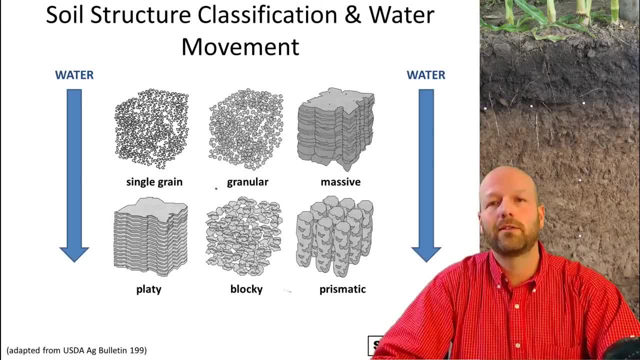 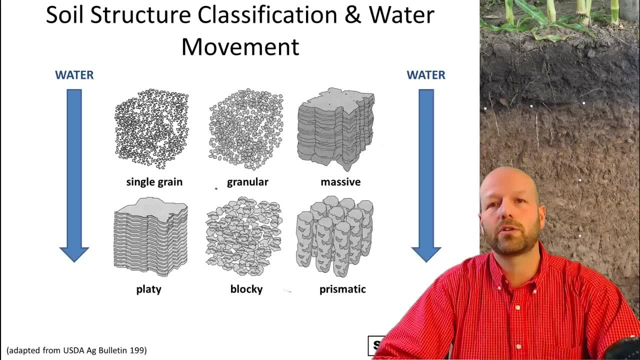 water. as you can envision, it's a pretty straight shot Water. we can flow through that fairly easily. So again, soil structure very important, Not only the particle size, distribution or the soil texture, but soil structure is extremely important for water relations in the soil. 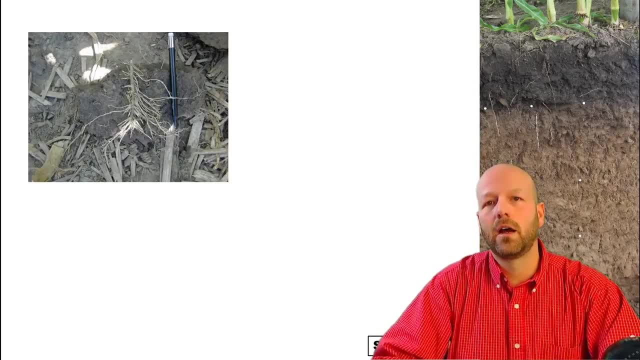 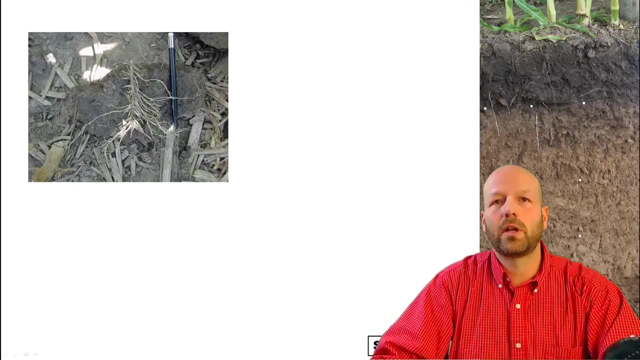 Here's a good example, too, how a structure can affect other growth parameters or crop growth factors. So you can see here this is actually a picture out of a soil out of Arlington At first. look you can see that, oh, there's some nice root growth through that soil. 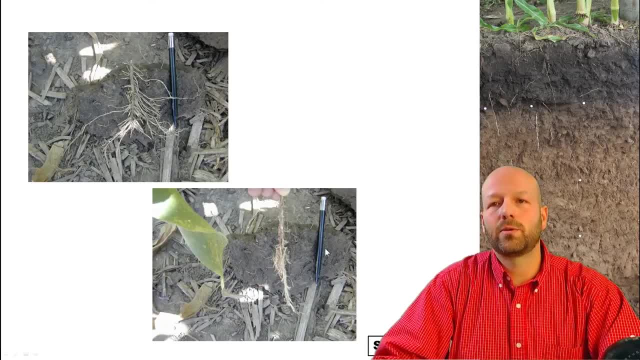 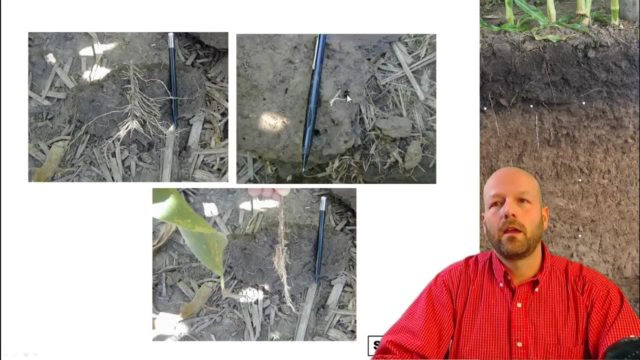 But if you look at that in more detail, actually there's a condition where the soil was compacted and you can see that root just growing really flat. So that's the same root that's been turned around And, even though you know, 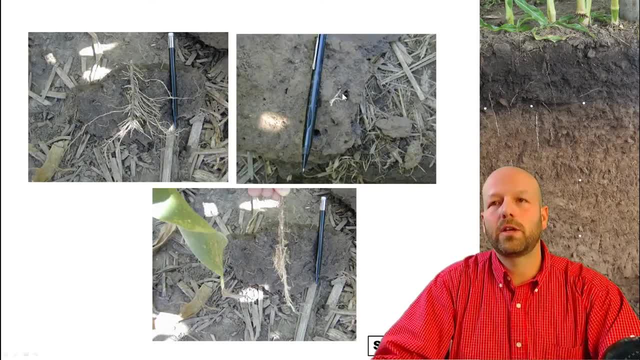 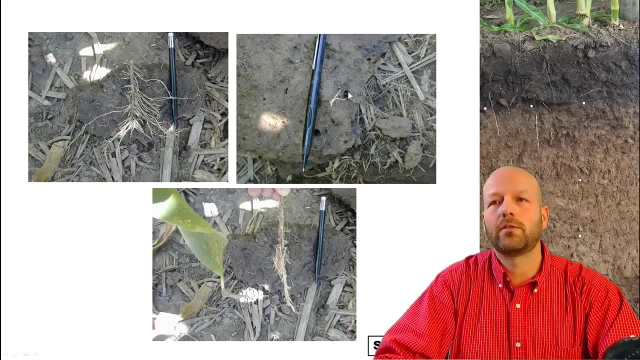 that soil is an example of compacted situation. sometimes you can still have macropores that are caused by biological activity, So in this case this is probably some kind of insect hole. You can see there's some organic matter that has flowed through it. 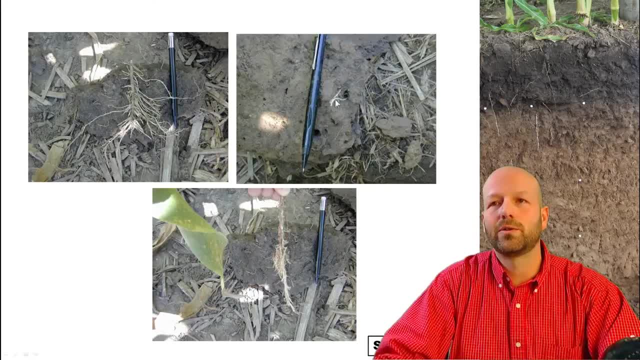 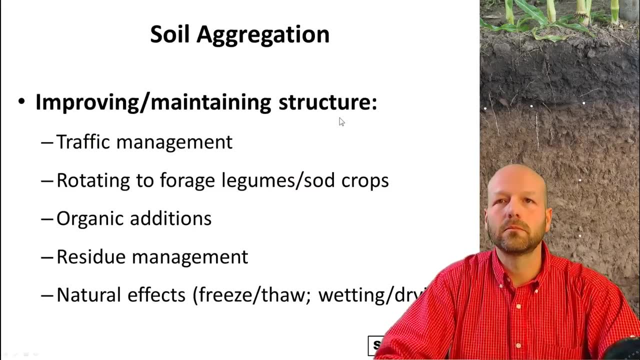 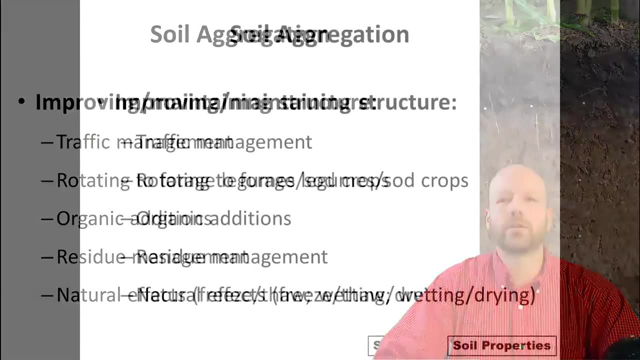 And you can see roots taking advantage of those holes, those macropores, to grow because they're having a harder time growing through the massive structure. So how do we manage soil irrigation? What factors affect soil structure? Obviously traffic. So anytime we put a piece of equipment in the field. 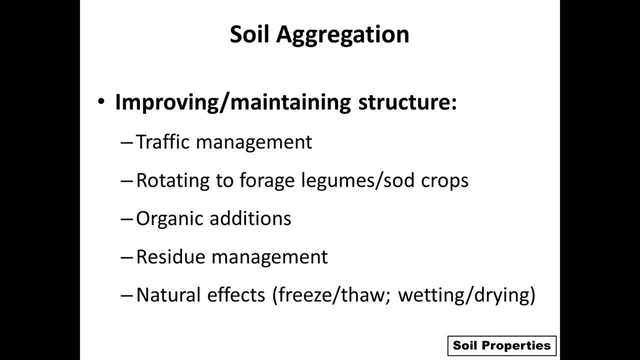 it will tend to crush those aggregates in the field, So excessive traffic could be a problem. We'll talk about this in more detail when we talk about soil compaction. Insect and health, for example, would be crop rotations would be very beneficial. 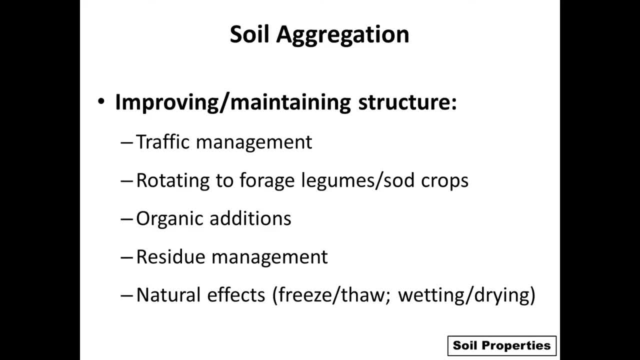 Addition of organic matter manure. So one thing I have not discussed is the impact or the role of organic matter in aggregation. The organic matter essentially works as a glue that sticks sand, silt and clay together, gives them stability. Obviously also then residue management. 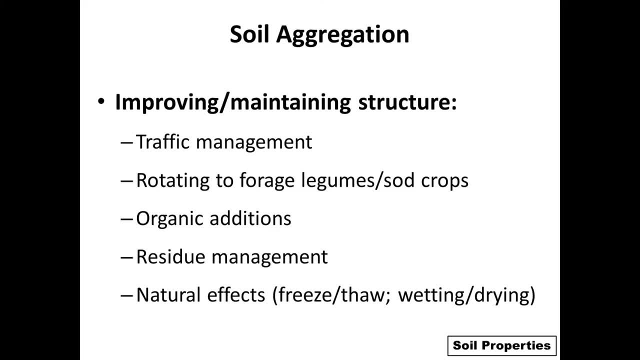 So anything that affects carbon in the soil or organic matter in the soil would be something that affects aggregation, And then, last but not least, also naturally the effects such as freeze-thaw cycles and then wetting and drying cycles. They have a similar effect. 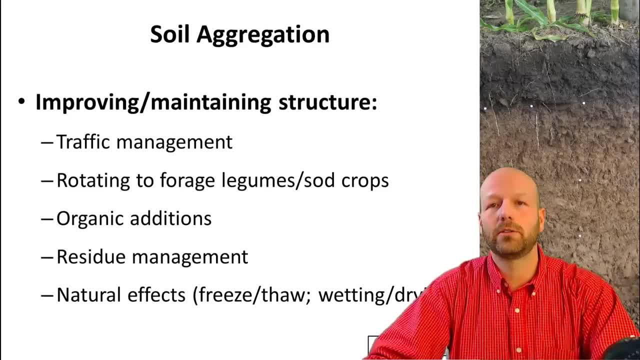 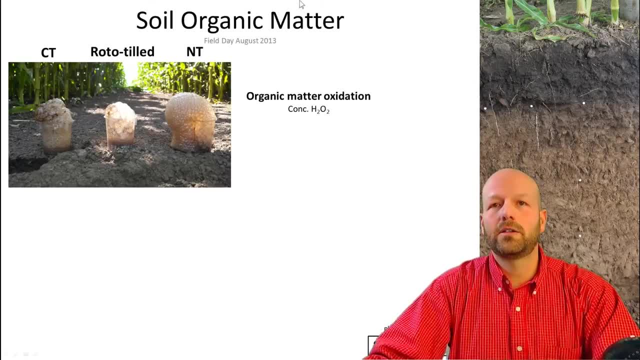 where the soil expands and contracts And so it helps that aggregate formation. So, talking about the importance of organic matter, I just mentioned that in a second. Here's an example of a little demo we did on a field day out of Arlington looking at a conventional tillage system. 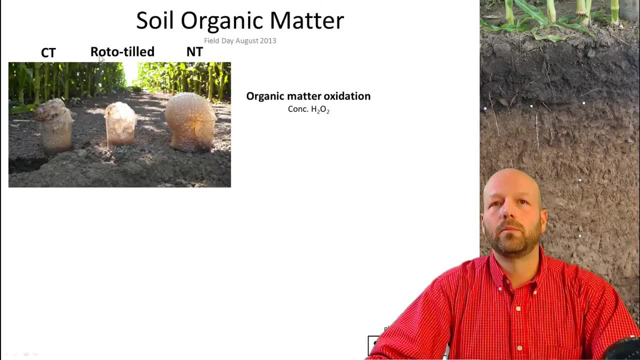 a no-till system and then a rototill And just kind of try to do this relative comparison of organic matter on these three tillage systems. So what we did? we added some concentrated hydrogen peroxide to the same amount of soil. 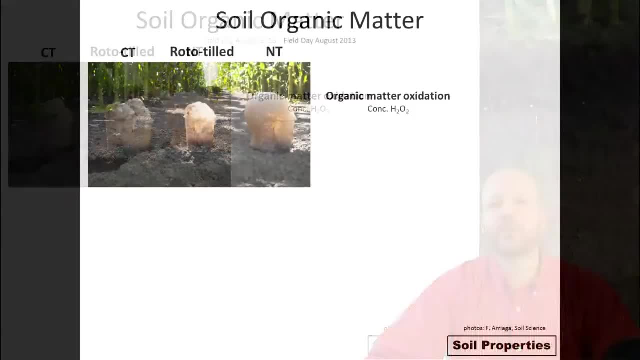 on each of those little cups and then looked at the aggressiveness, if you will, of those reactions. So the more organic matter, the more fissing you would get. And you can see in the no-till. you can see there's a lot of bubbles. 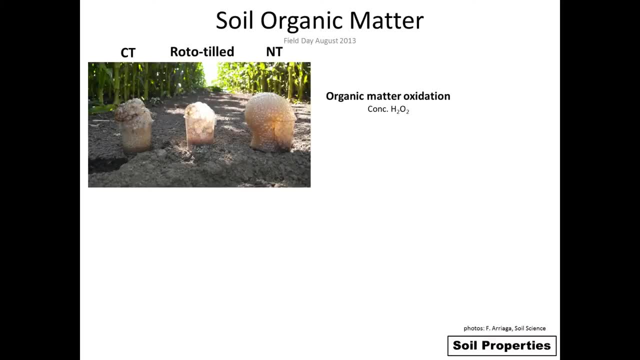 a lot of fissing that happened there. Conventional till actually didn't do too bad. These soils in Arlington are quite good, quite productive and have a high percentage of a high organic matter content. They are silt loams after all. 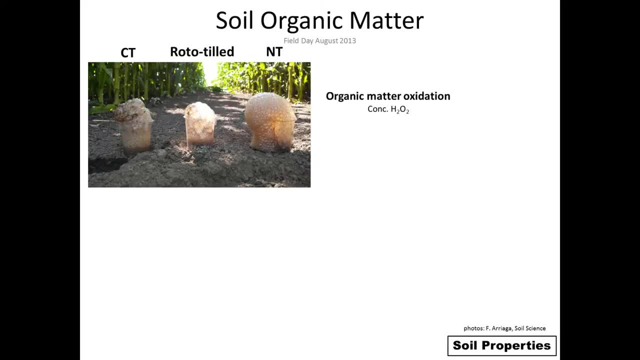 so they're very good at holding water in those type of things and very deep In the rototill situation you can see that that soil has a lot less organic matter, even though I was quite surprised that we got that much fissing. 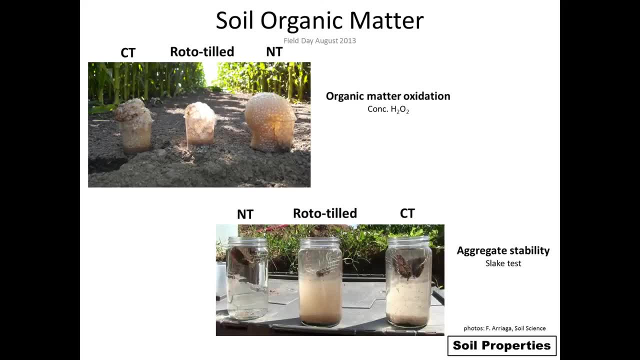 Again, those soils are excellent soils too. We also did what we call a slag test, And so that's just a way of comparing the stability of soil aggregates, And so what you do is you get a soil aggregate and you put it in water. 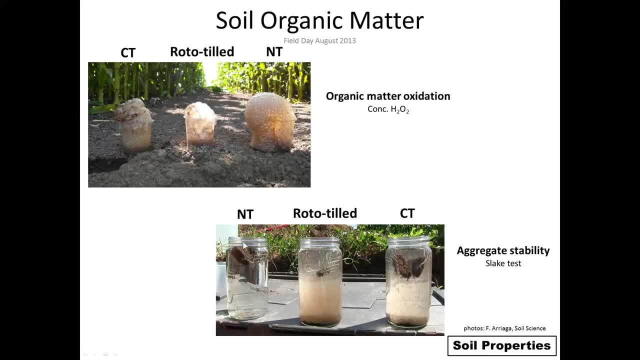 in a container with water. So in this case again, we have on the left the no-till, middle the rototill, and on the right the conventional tillage And you can see by looking just at the clarity of the water, that very few particles. 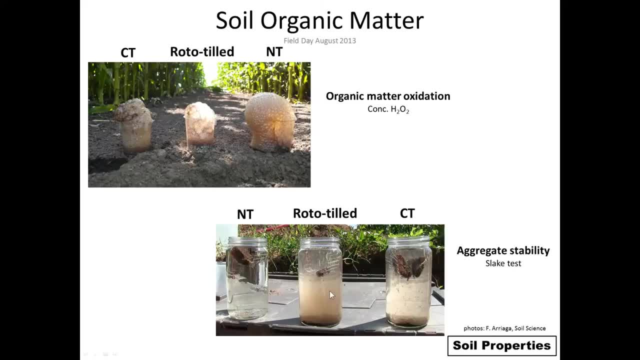 have broken off of the aggregate from the no-till scenario. The rototill almost completely has disintegrated, no structure whatsoever to it, very, very, very weak strength And then the conventional tillage. not too bad actually, but you can see that it's not. 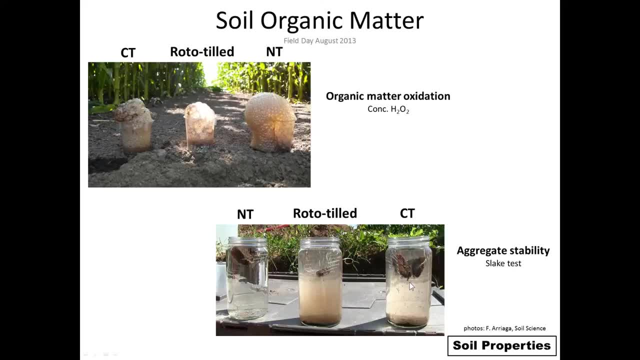 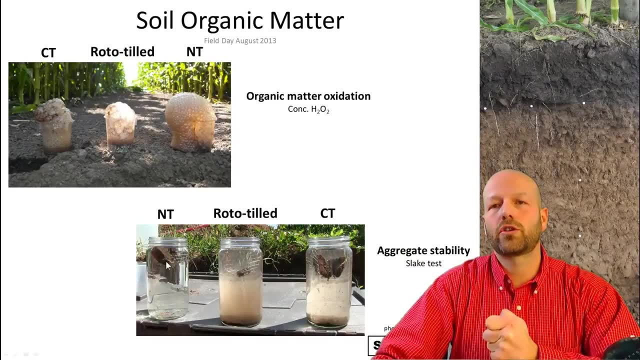 as stable as a no-till. So if you imagine a raindrop impacting the surface of these soils, the soils with the stronger structure, stronger stability, are going to be able to stand that a lot better than soils that have a weak structure. 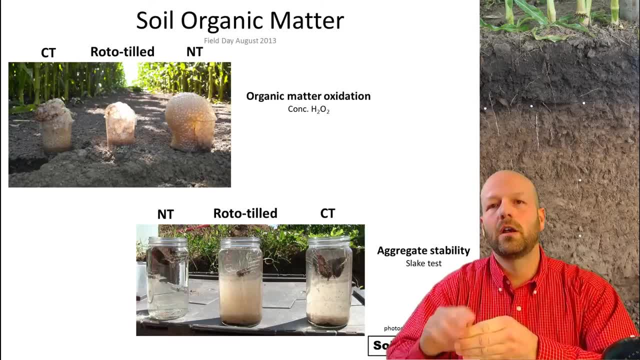 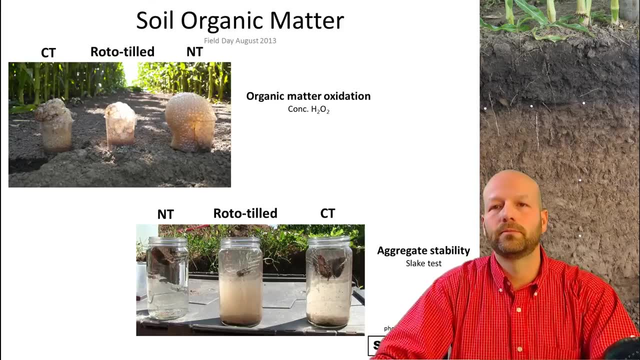 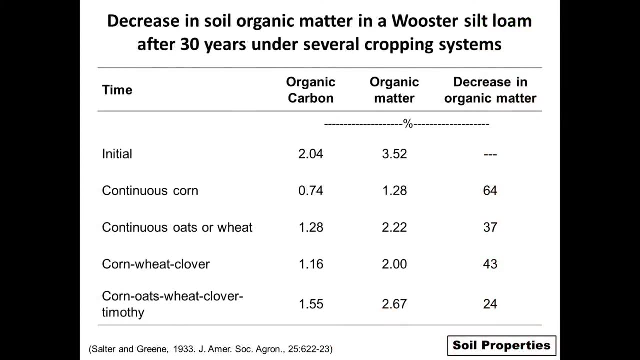 So those soils that have a weak structure are going to tend to crust a lot easier and then that's going to cause problems with inhibiting infiltration and eventual erosion problems. So we know that other things, not only tillage, affect also organic matter accumulation in soil. 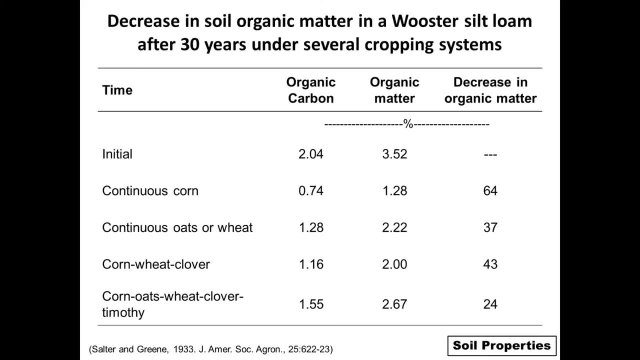 This is information or data out of Ohio, And so we're looking at, after 30 years, different cropping systems. So this is the initial on the left: continuous corn, and then a continuous oats and wheat or wheat system: corn wheat, clover and corn oats. 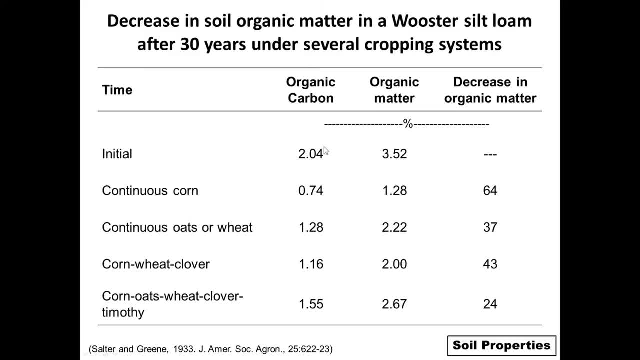 And we can look at the original carbon content was about 2%. That translates to about 3.5% Organic matter. if you think that way- Continuous corn- you can see there was a big drop. So it's a 64% decrease in organic matter. 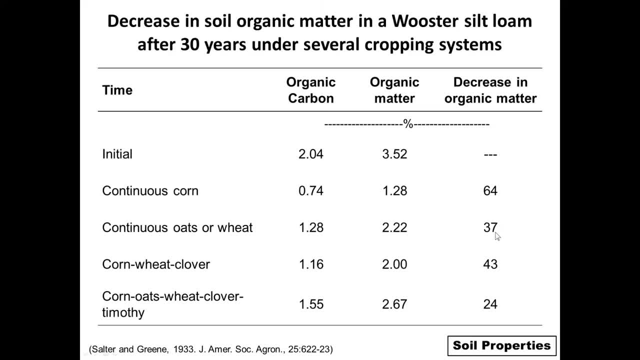 Wheat or oat decreased about 37% from the initial 43% decrease. when you were on a three-way rotation- corn, wheat and clover, And then on the bottom rotation- you can see that the decrease was only 24%. So the point here is that 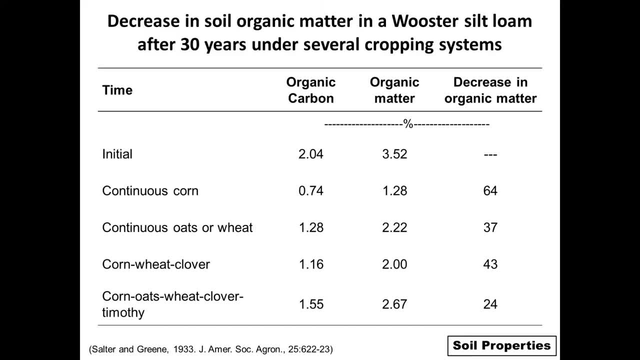 every time we manage soil or we manipulate soil we're going to cause any soil disturbance. We will be losing some organic matter. However, we can actually try to reduce that and maximize the amount of organic matter that we have in the soil through management. 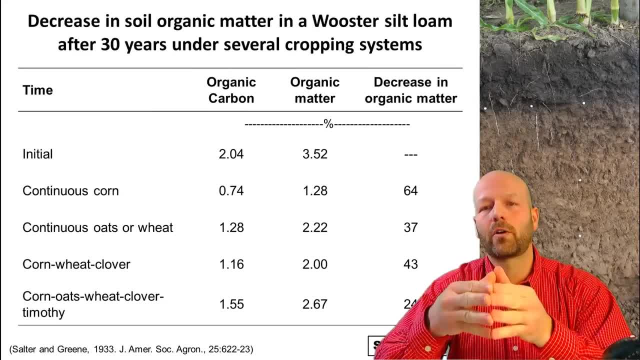 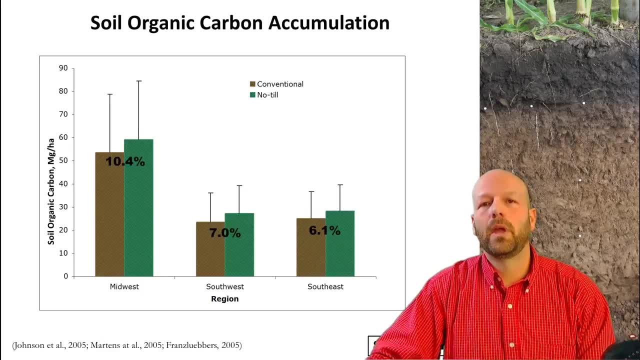 So either tillage or rotations, additions of manures, use of cover crops, all of those are tools that we have in the toolbox that we can use for proper soil management. Another thing I wanted to highlight is that there is a difference in organic matter accumulation depending on regions. 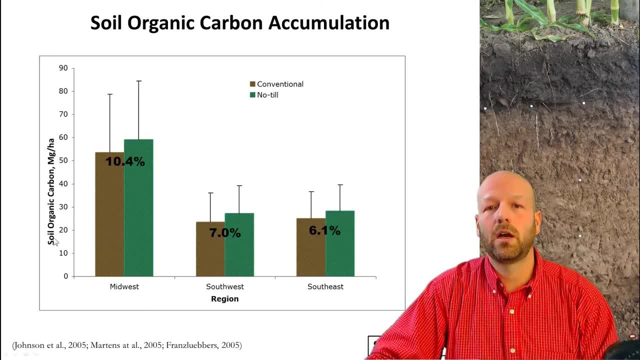 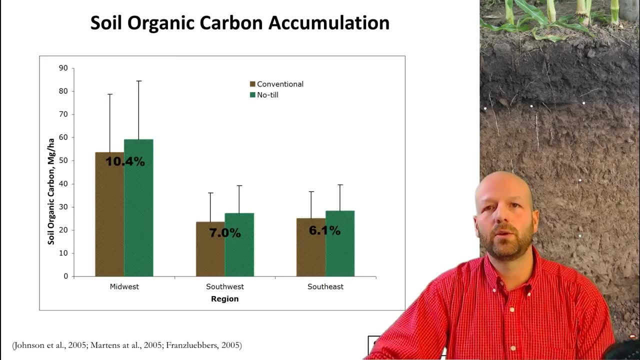 In this case we have a solar organic carbon accumulation And this is compiled from several studies that looked at a lot of different studies. in general in looking at organic matter accumulation, mainly looking at tillage, conventional versus no-till. The no-till is in the green. 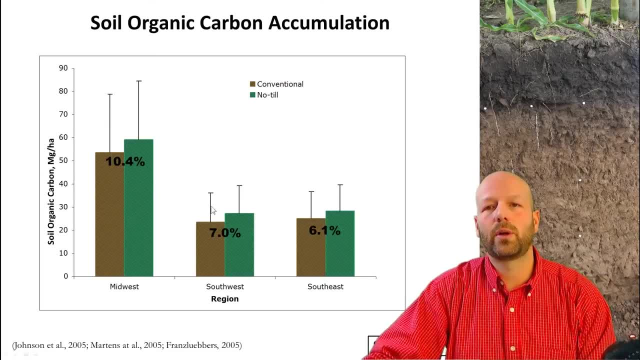 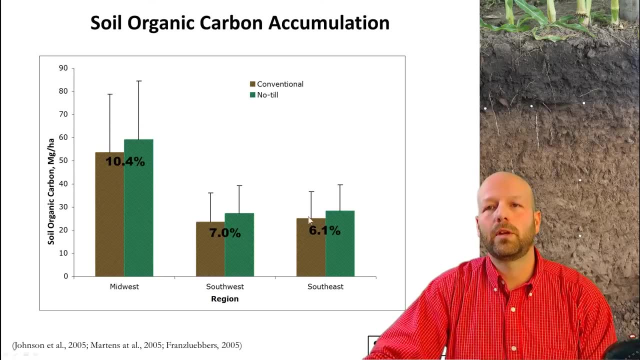 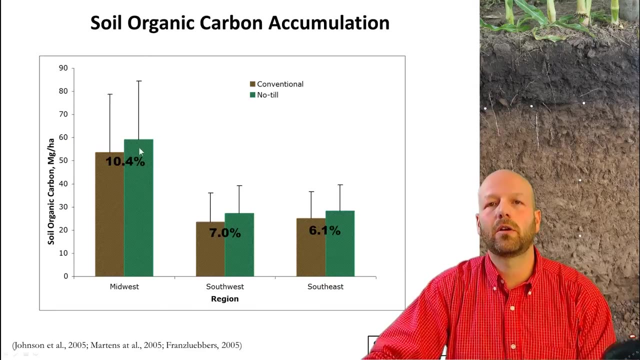 conventional in the brown. We can see in the Midwest, compared to the Southwest and the Southeast, we can accumulate a lot more carbon overall. Looking at the size of the bars, we can see with the no-till in all three regions we can accumulate a lot more organic matter. 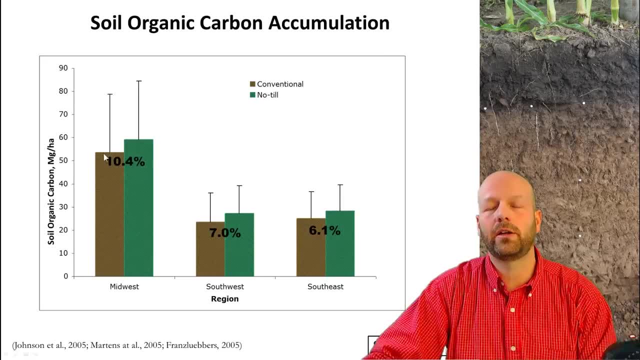 And the other thing that we can see in each region: comparison of the tillage system. so the conventional versus the no-till. on the average the no-till accumulates about 10% more organic matter In the Midwest and the Southwest, 7%. 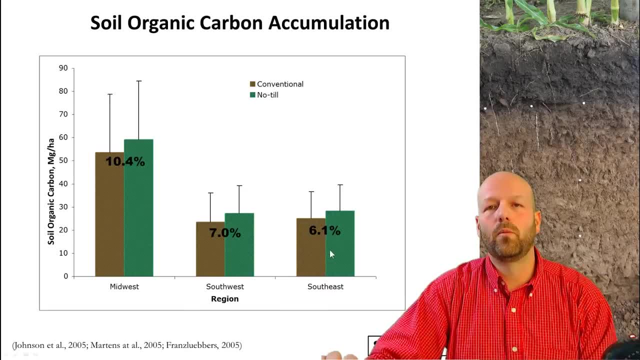 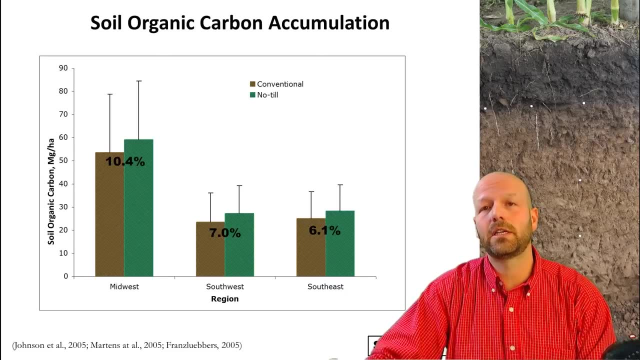 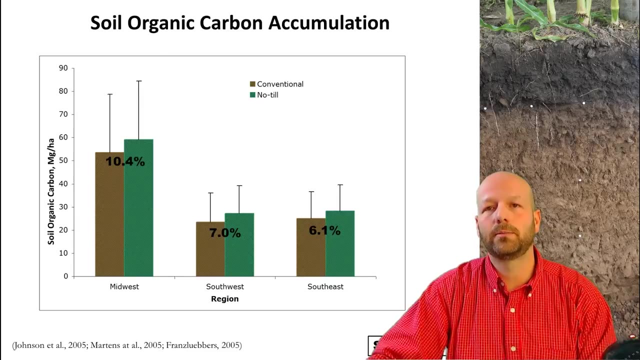 In the Southeast about 6%. So the reason I wanted to share this with you is to basically highlight the importance of climate difference in climate between regions and then also differences again on management. how can that impact carbon accumulation in the soil? 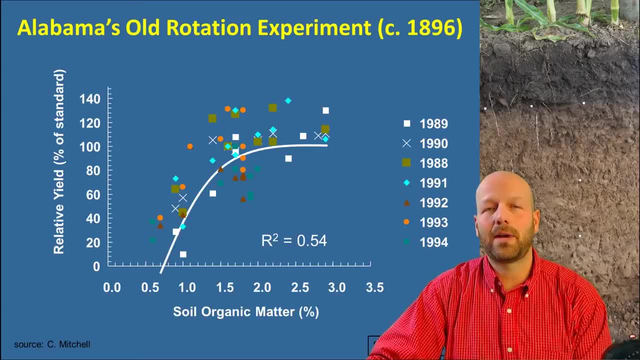 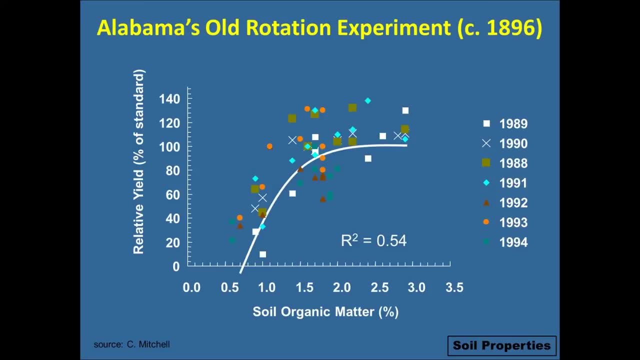 And here's another good example. This is actually from Alabama. This is from the old rotation experiment. It is the third oldest agricultural experiment in the US and it's the oldest continuous cotton experiment in the world. It was established in 1896,. 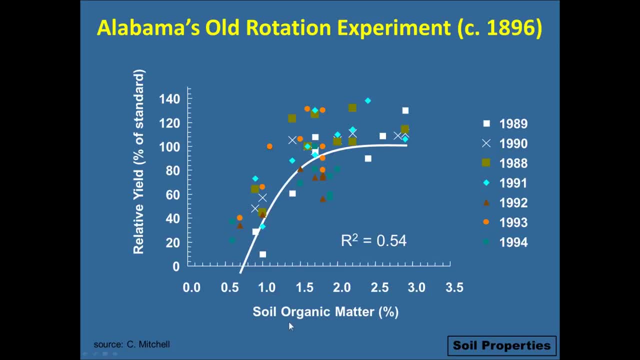 right there on the campus of Auburn University, And so what we're looking at here on the bottom is solar organic matter and on the vertical axis is actually the relative yield. So this experiment has about 12 different management systems looking at rotations in tillage systems. 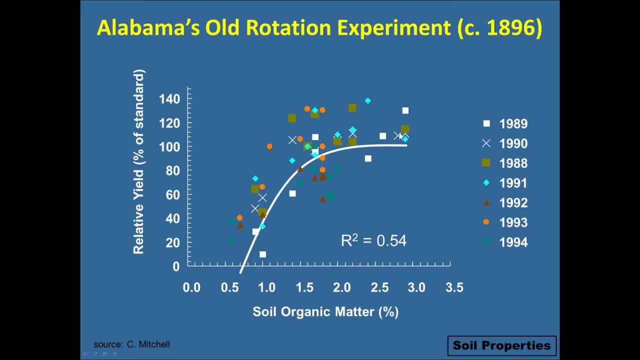 And what we're looking at here is different samplings from different times- so from 89 all the way to 94, and looking at the organic matter and the relative yields for those years in those systems in here And what we see is that we see an increase in yield. 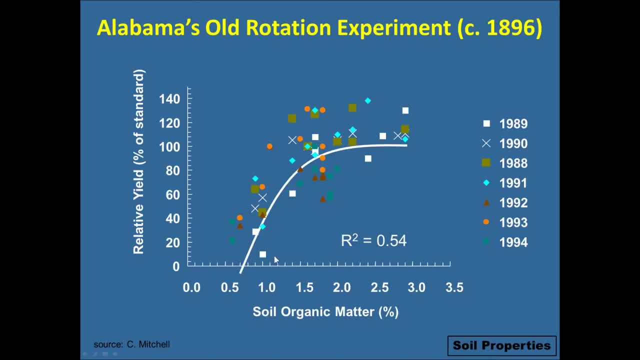 with an increase in organic matter. One thing that you might note here is that these soils being again the climate, like I talked before, regional differences and soil differences very low to begin with, and so a 2% increase in organic matter. 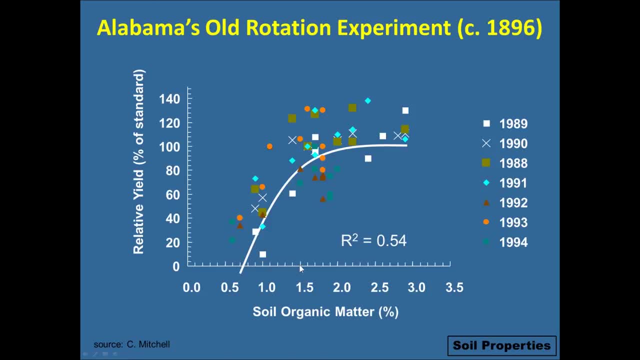 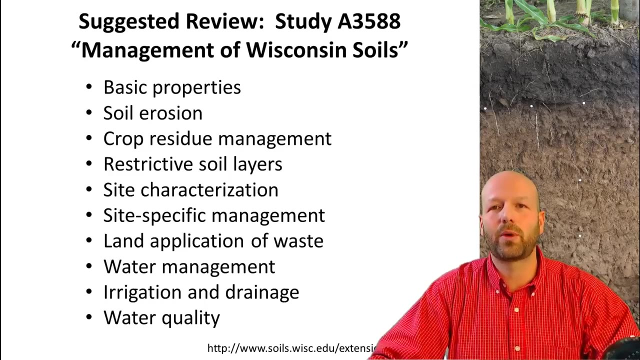 has a tremendous impact in yield in these type of soils. Similarly, we could probably realize- maybe not such a dramatic increase for our conditions in the Midwest, but we would realize some benefits from organic matter accumulation. This concludes our section on basic soil properties.